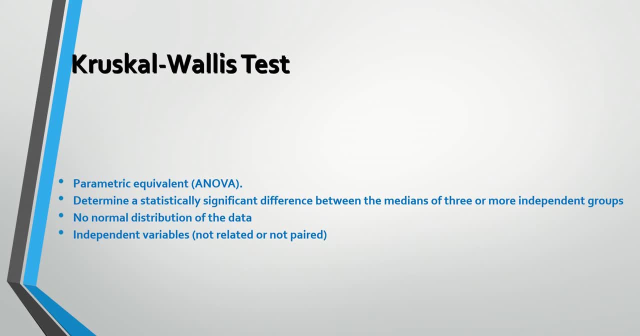 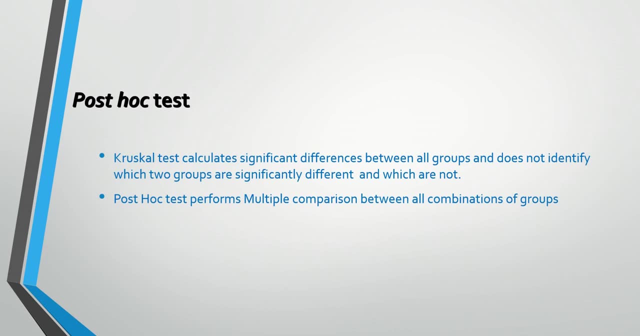 the data are not normally distributed and the groups are independent. they are not paired, they are not related. now, what is a post hoc test, as we know that? as it's known, kerscale test calculates significant difference between all groups and does not identify which two groups are significantly different and which are not. 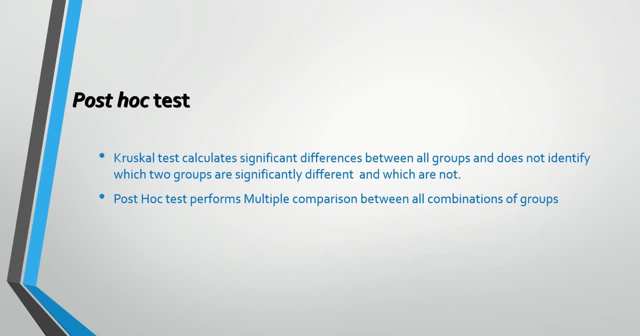 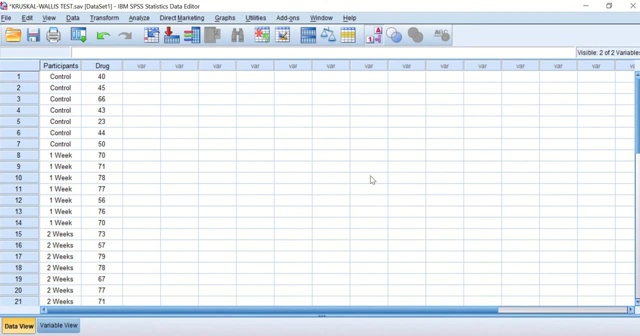 post hoc test performs multiple comparison between all combination of the group, so we'll go to the sbss. in this data view i have three group group number one, which is a control, two is the one week and three is two weeks. so these, through three groups, a drug. 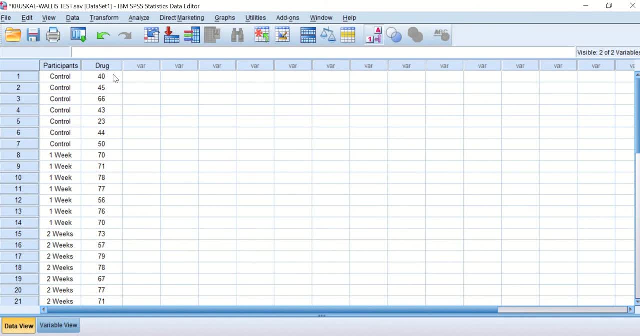 new novel drug has been designed and its effect has been followed up using uh specific parameters in the blood. so we want to compare the efficacy of the drug um after using it for one week and two week, compared to a control. again i've double checked the uh distribution of the each group. 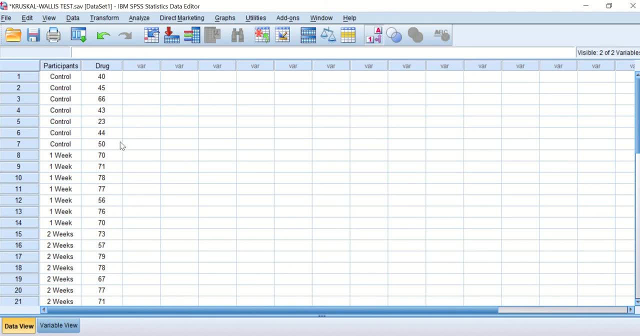 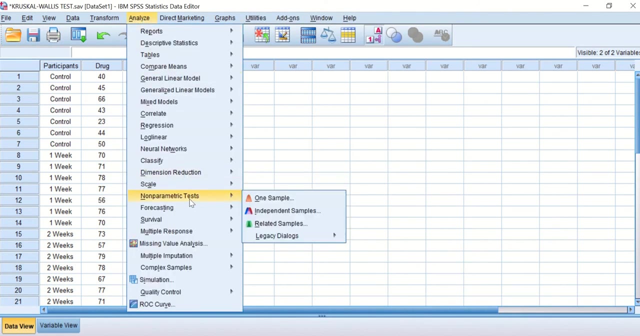 control week one and week two and they are not normally distributed. so how can we do kerscale wallace test to determine the significance, whether there is a significance between these groups? look and analyze, scroll down to nonparametric test and then to legacy dialogue and then we click in the on the icon for k independent samples. reset this, okay. 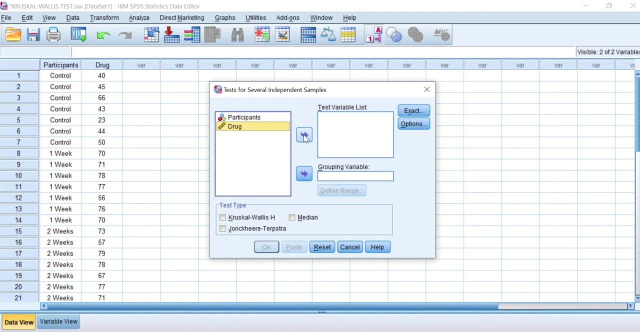 so i'm going to transfer the drug into tested test variable list and the participant into group variable and in the participants, i want the range to be from group number one, in which i gave the control value one and uh um, to the week two, which is value three. 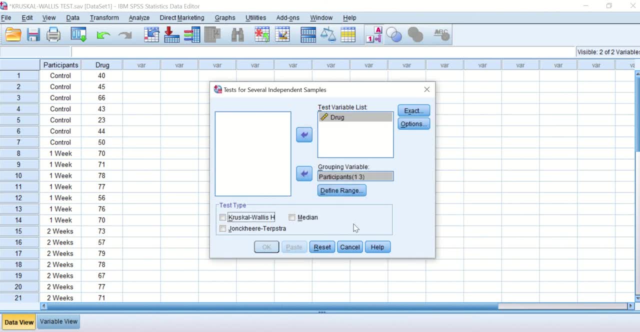 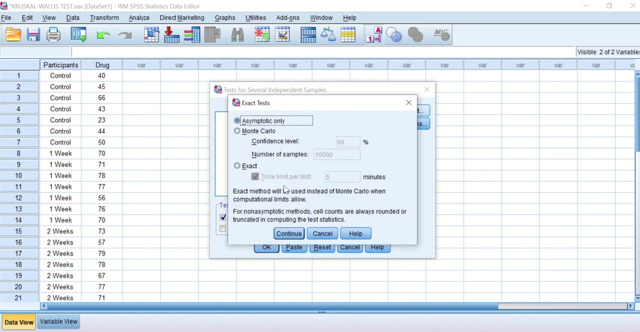 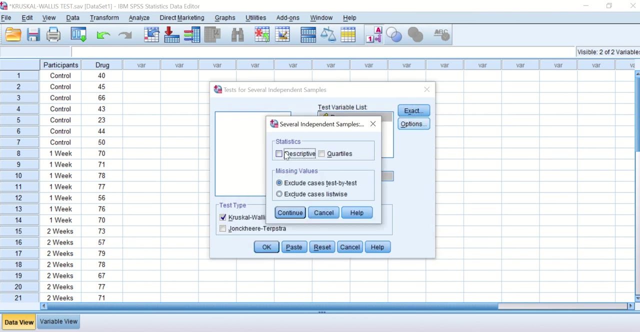 and week one is value two. click on continue. click on the icon for cascal wallace and then check on. click on exact. we'll leave. our new window will appear. we'll leave the symptomatic or asymptomatic only test as it is. click continue on the options. we will just click on the descriptive and then. 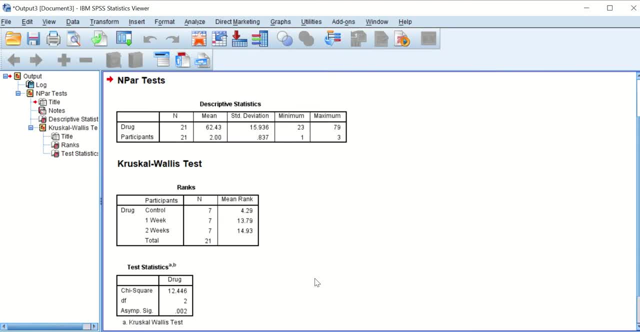 we click continue. hit the button for okay. spss will produce these tables. the, as it says here, 21 participant involved in this study and out of these 21, seven were controlled. seven week uh drug has been given for one week and two week or two weeks. and what has uh this? 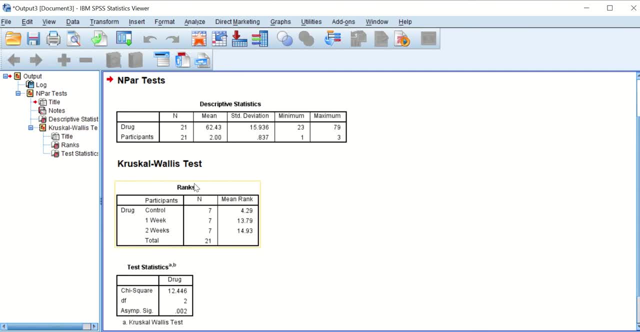 cascal wallace test. done is put. took the actual data for each one of these and sort them into ranks and then calculate the meal rank and we can see from the meal rank that control compared to week one week is. really there is a huge difference from 4.2 to 13 and from control to two weeks is 14, also from 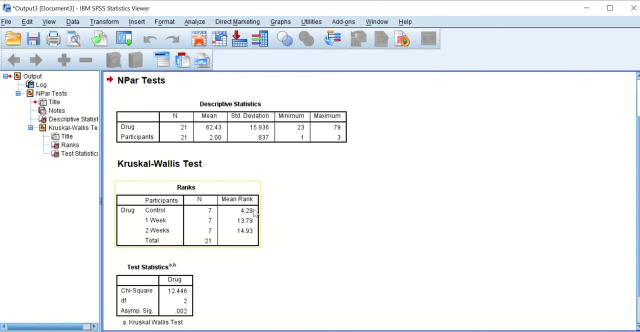 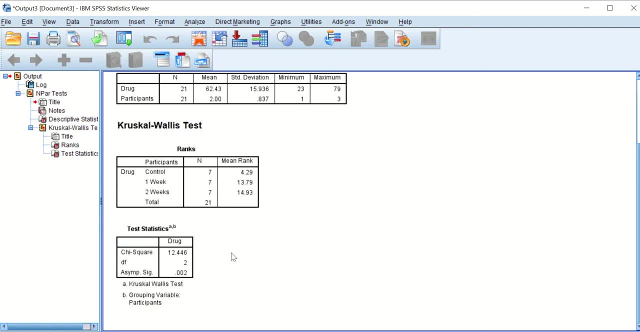 4 to 14.. however, there is no big difference between the mean rank of week one and week two. the test produced a significant value p value and the p value is is is lower than 0.05, which really indicate that there is a difference between a patient who or in or valon, or individual participant who has 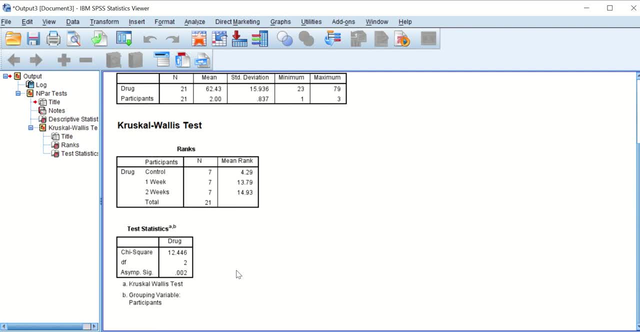 taken the drug for a week compared to control, or two weeks compared to control, and. but it doesn't tell you if the the difference where there is a different, significant difference between the control and the week or the control- uh, week one or week two, or week one or week two. it just gives you a p value. 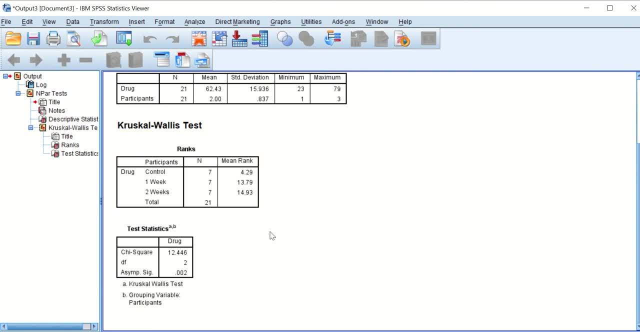 for all three groups. and now to nail down this into which groups, which two groups really are significant, which are not, as i see i showed you in the previous um video clip. you can go do, man Whitney. you test on two samples: control on week one, control on weeks two. 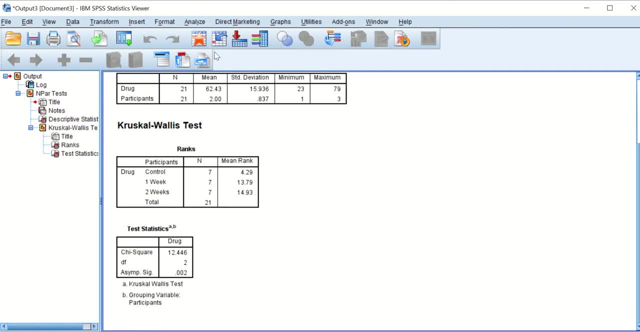 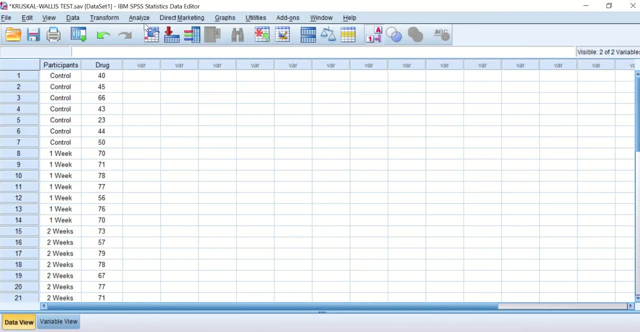 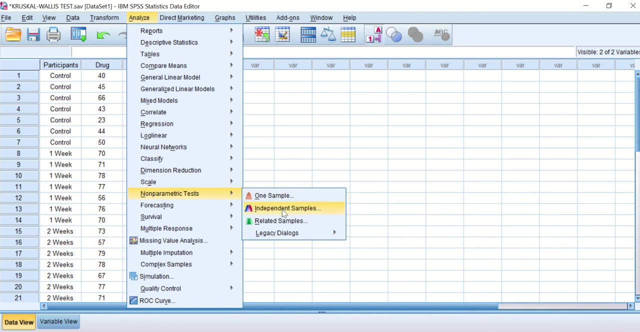 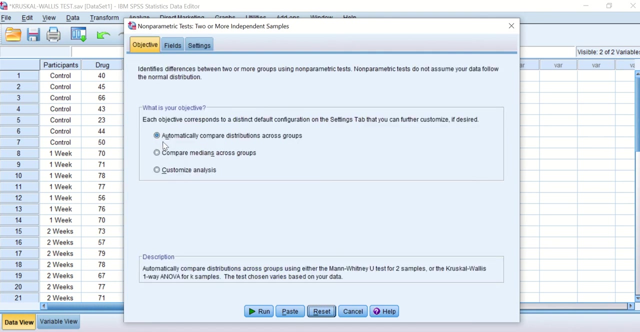 two weeks and weeks one and week two. however, there is another way to do it, which is called post hoc test. to do a post hoc test, I'll go click on analyze, scroll down to non-parametric test, click on the independent samples, click reset here objective. so in this icon, in this sorry window, I will appear and ask you. 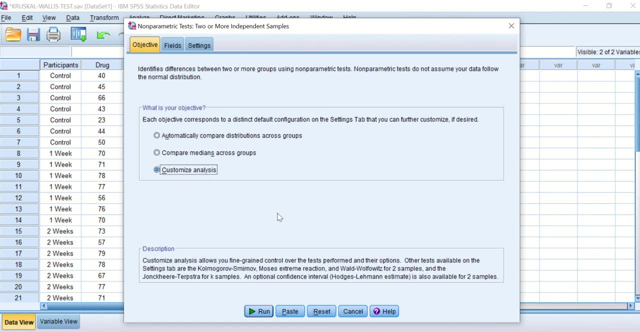 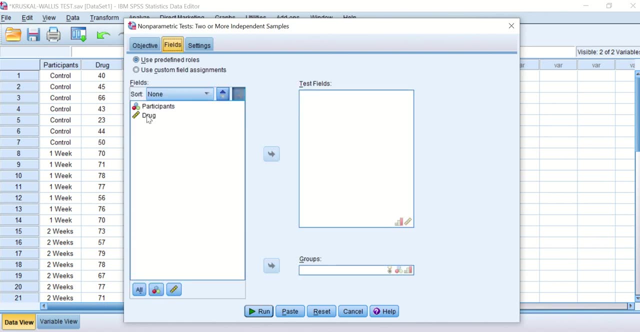 what is your objective? say I wants to customize the analysis. I want to what to do, to tell the software what to do, click on there in the field. I'll transfer the drug into the test field and the participant into the groups and then in the last icon here is the settings. so what I want to sort to the sitting I 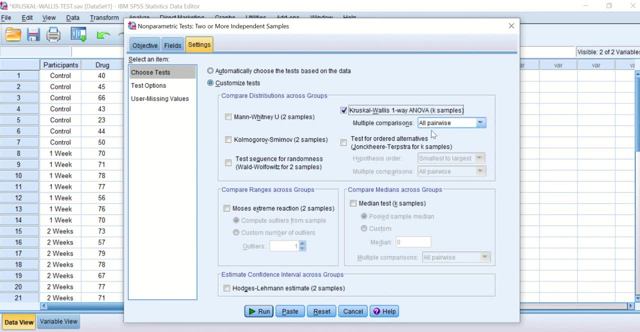 will select the test field and then I will select the test field and then I will click on customize test and I will click and care scale willis one way and it automatically says: do multiple comparison pairs all pair wise. so it will do a pair wise between control and week one, control, week two, week one and 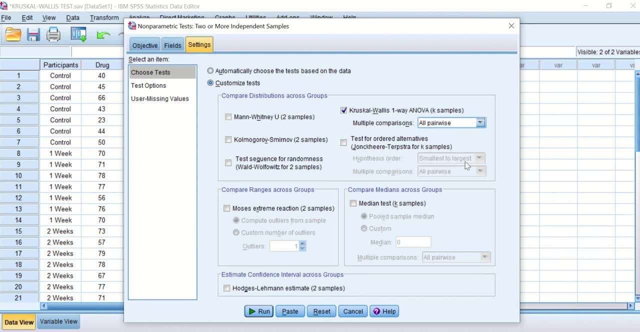 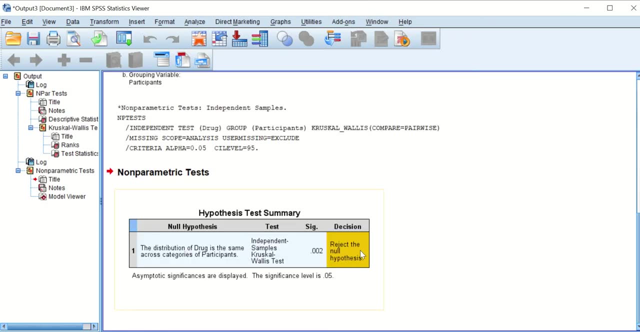 week, two weeks, two together or two weeks together. so I'll hit the run and then a table, small table, saying here that the hypothesis test testing that there is a difference between the three groups and the difference is 0.002, and to find out which groups, which two groups, really have. 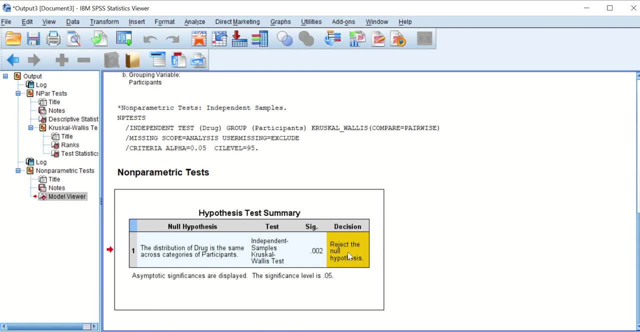 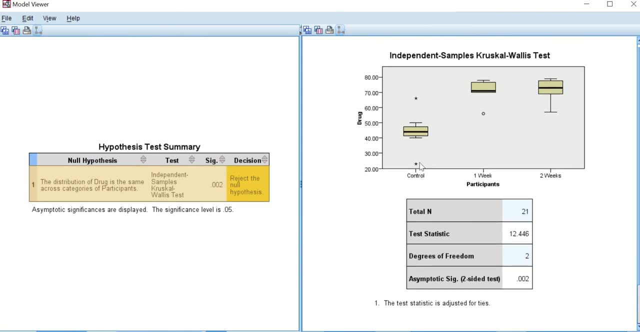 a significant value and which are not. double click on the table and then another window will appear showing you the box plot for control. one week and two weeks. as you can see, there is not that much difference from this diagram between one week, one, one week and two weeks, but there is really a. 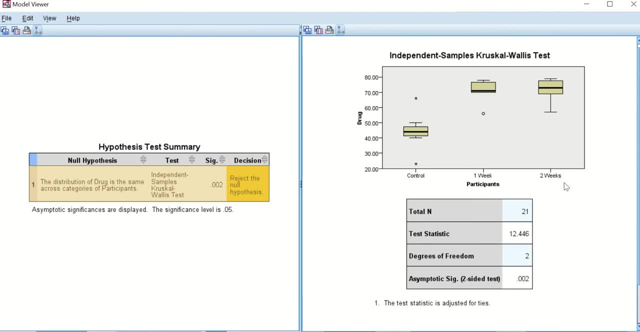 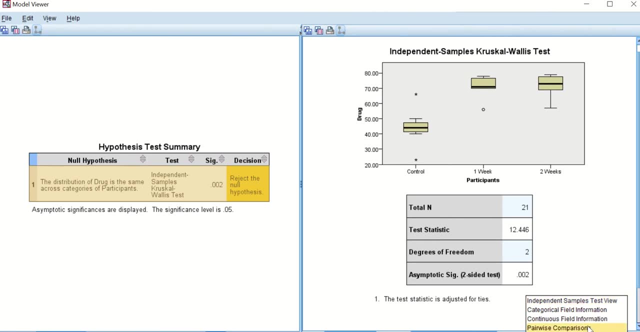 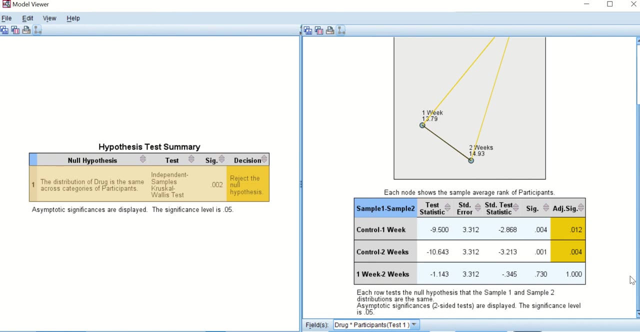 difference between controls and week one and weeks, week two weeks to do, to, to do. and then we click in another one called bears, wise comparison. that's a table will appear here. that's the table that will really do the comparison of control one and week one week and it's give a significant value of 0.012 when a test. 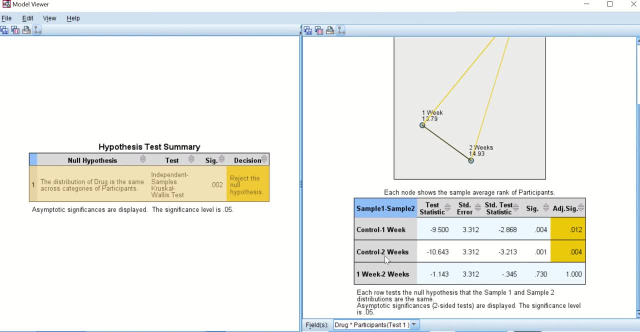 has been done to between control and week two weeks, it's give less than 0.05 significant. however, when we compare week one with week two, there was no significant. the value was one. so this table tell you, Chris Calvallis, tell you, that there is a significant difference between all the three groups. this table